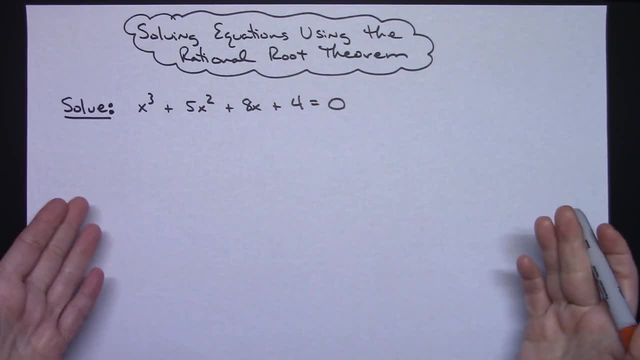 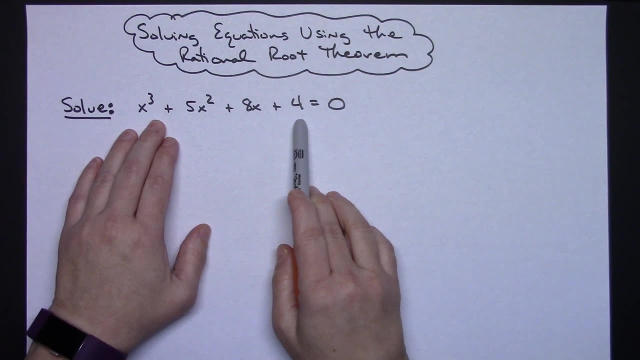 Okay, in this video I'm going to take a look at how you would utilize the rational root theorem if you were trying to solve an equation. Alright, now, if your equation has four terms and you're not sure how to go about solving that, the first thing you should probably always do is try factor by grouping and see if. 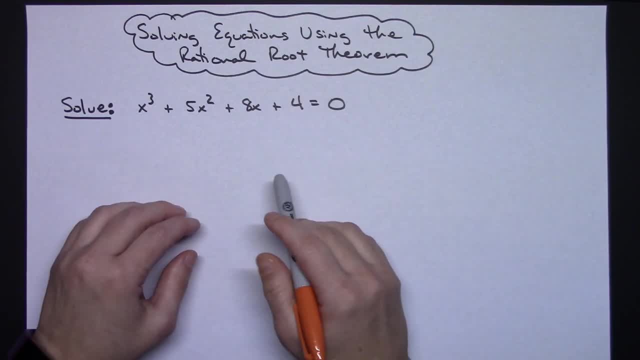 you can factor this into two products, Alright, set equal to zero. and then you could use the zero product rule, zero product principle, and set both of them equal to zero and solve Alright. but if it doesn't do factor by grouping, then you're going to have to try something else. Now the rational root theorem does. 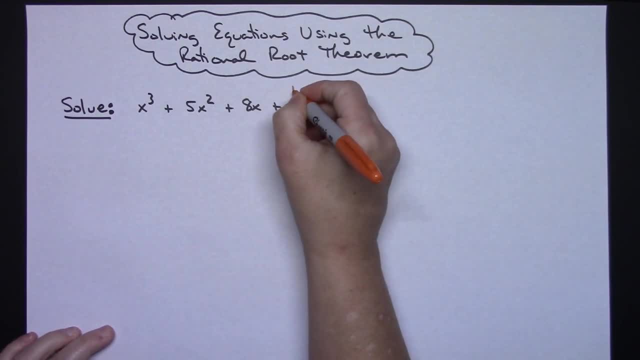 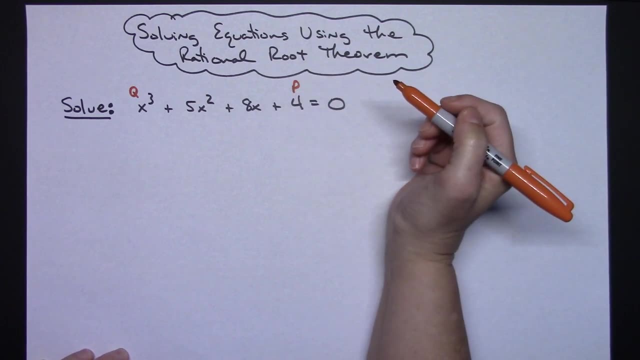 a thing with P's and Q's. They usually call this P and they usually call the coefficient here Q, Alright, and then you do plus or minus all your factors of P over Q, Alright, and that will be one of. those are hopefully going to be a root. 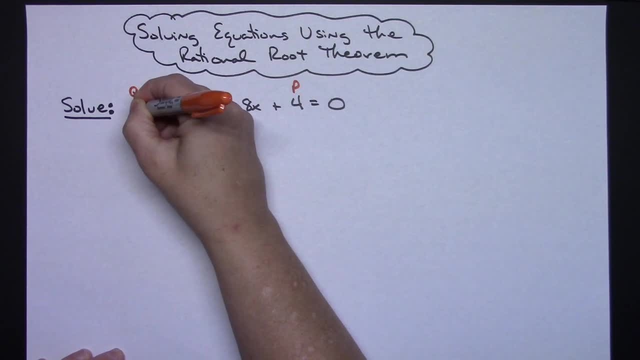 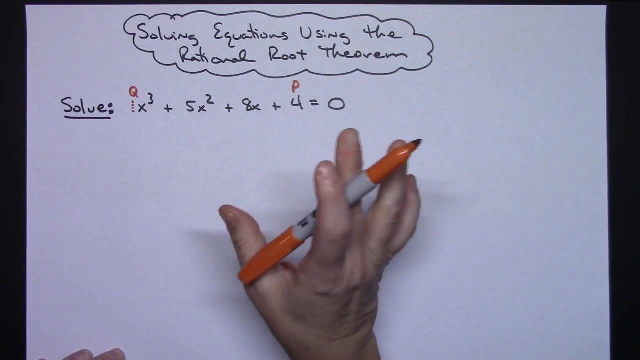 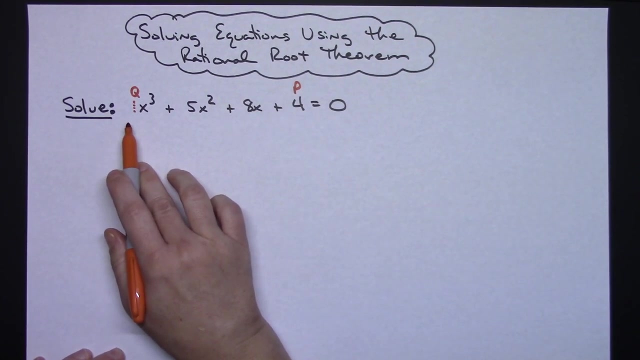 of the equation. Alright. now, in this example, my Q is a one, Alright, and if there's a one leading coefficient right there, then it makes it really, really simple. because P over Q, all your factors of four over all your factors of Q, Well, with that being a one, then we don't really need to deal with. 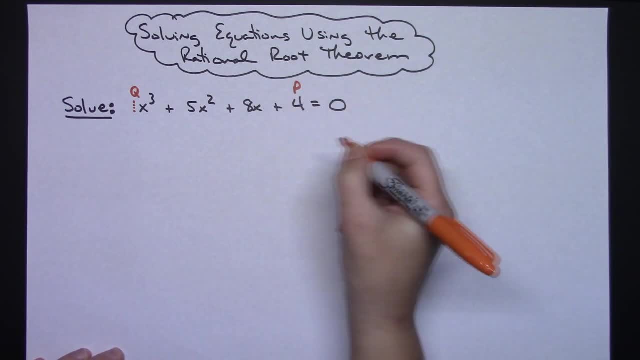 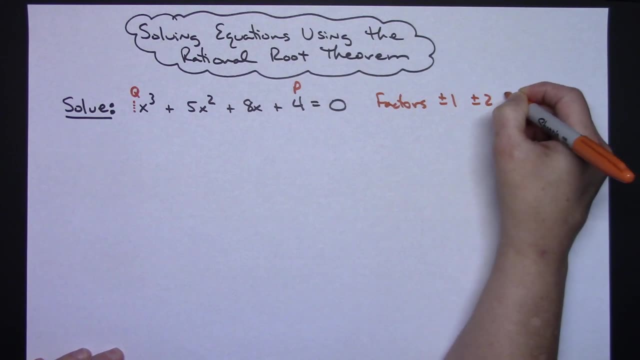 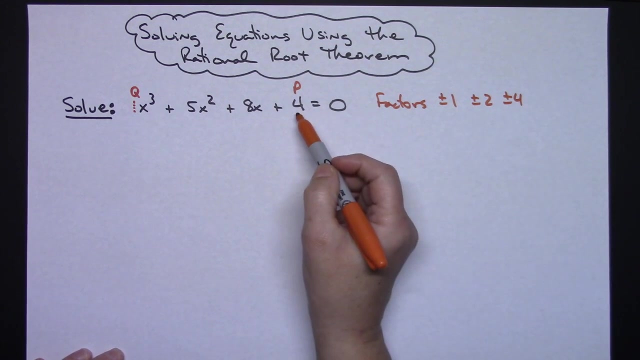 that at all. So really, in this case, on the four here, the only factors that we are needing to deal with would be plus or minus one, plus or minus two, plus or minus four. Okay, so those are not very many things to try. Now, what the problem here is: you've got to figure out which one of these work to go. 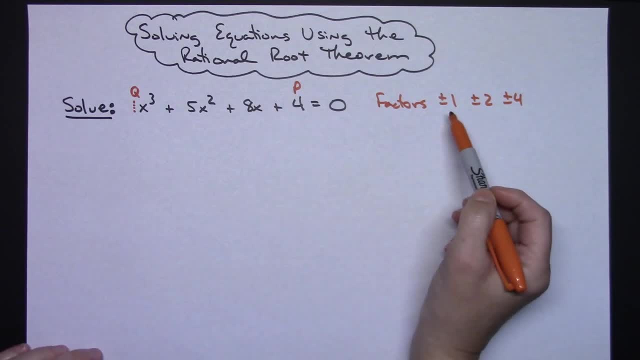 and solve this equation Now, the easiest way is to test one of them and use synthetic division. Now, generally I do not ever try the plus or minus one because it's trial and error. So the quicker you find it than the quicker this process is going to go You. 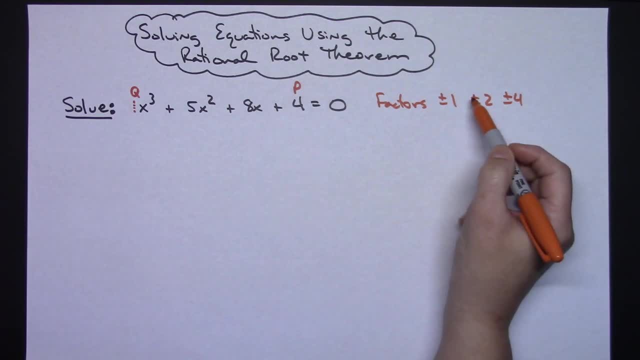 know you could try one and it not work. You could try negative one, that doesn't work. You could try to and it doesn't work. so you have to literally try each one of those. So when I start my guess and check process, I don't ever try plus or minus one. 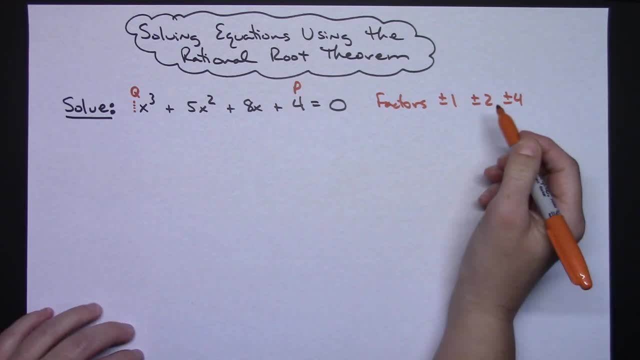 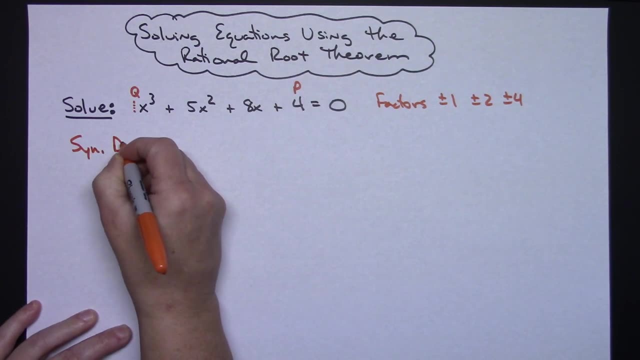 I always go to the next one. Alright, in this case, I don't know, let's try a negative two. Alright, so I'm going to use synthetic division. So let's go synthetic division to test factors. Okay, so that's what I'm going to do. 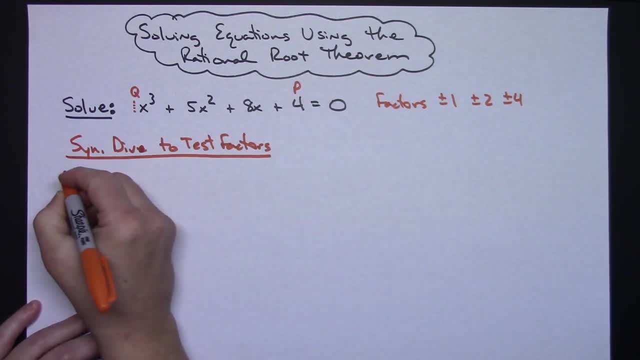 I'm going to use synthetic division to test my factors, Alright, and then I'm going to try a negative two, because I really think that one works on this one, Alright. now synthetic division Coefficients out of here. So one, five, eight, four. 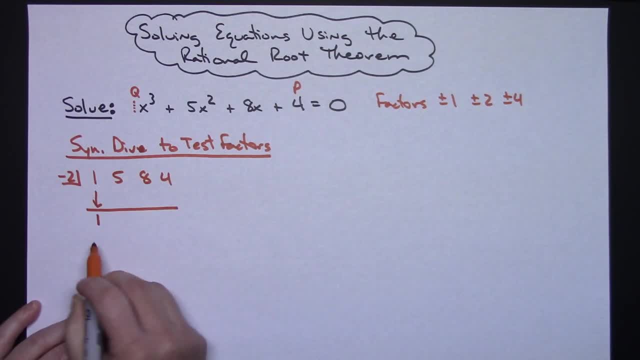 Okay, if you remember this, one comes straight down, Alright. and then two times negative, one is going to be a negative two. You add going down, So five plus a negative two is going to give me three, Three times negative, two negative six. 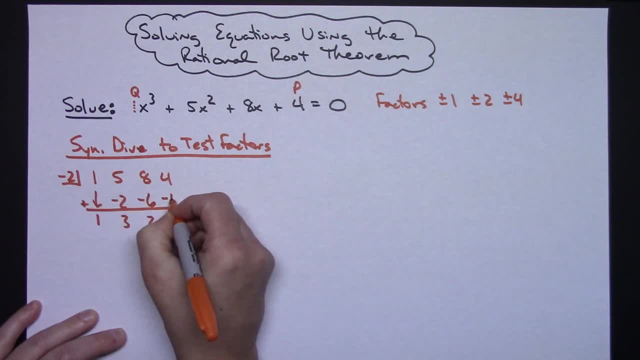 Add, coming down, I get a two. Two times negative. two is going to give me a negative four. Okay, so I'm going to use synthetic division to test factors And then I get zero when I add going down there. Alright, now that right. there is the key. 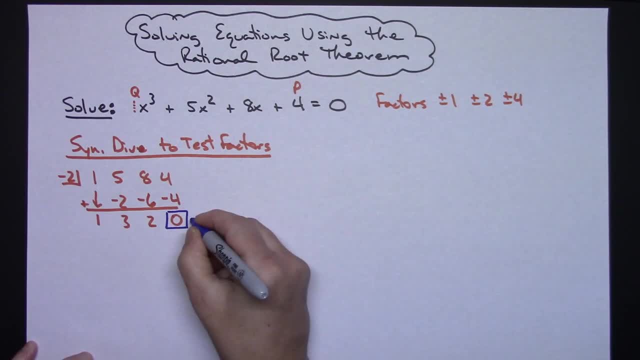 We want a remainder of zero. Okay, that is a remainder of zero, Because then if I get a remainder of zero, then I know that I've got a factor. Okay, so your trial and error process would come into play if you tried, like say four, and it doesn't work. 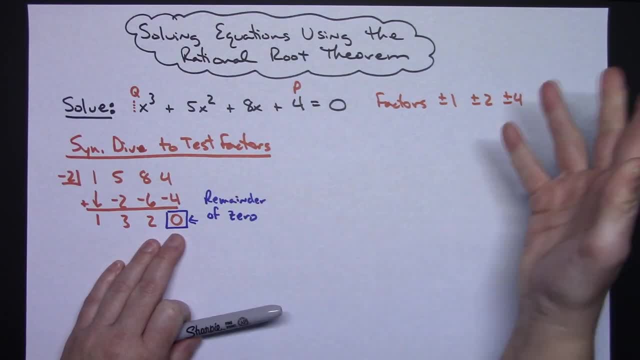 You don't get a zero there, Then there's where that tells, Okay, I've got to try something else. If you tried the negative four and it didn't work, you don't get a zero here, then it's not a factor. 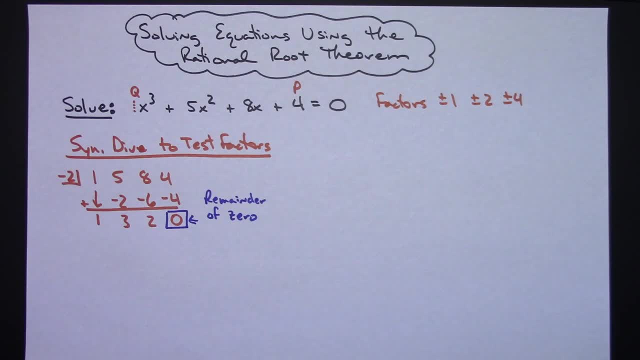 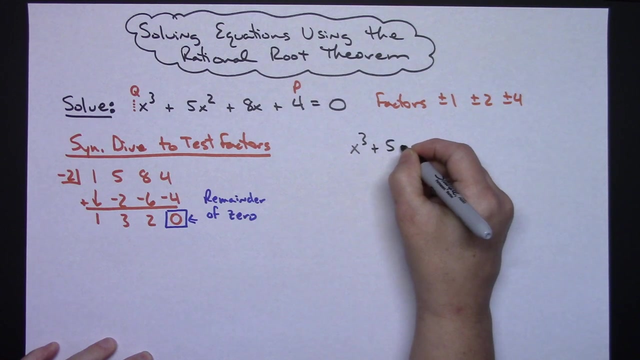 So then you've got to find a factor, Alright now, from this. this is going to help us factor that original equation. Alright, so let's do the original equation here. Let's go back to black here. Alright, x to the third plus five x squared plus eight x plus four equals zero. 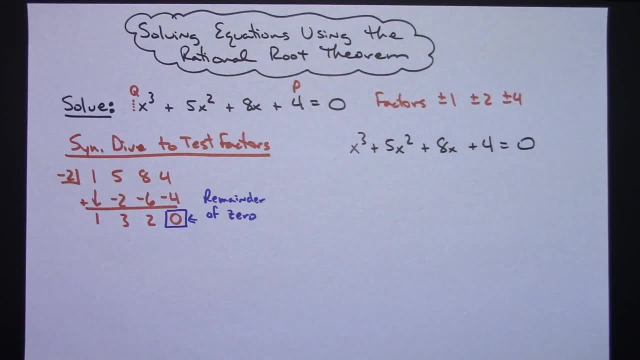 Alright, now this This is going to help us factor this. Alright now. what this tells us, right here, is that x plus two is a factor. So x plus two has to be a factor, because I've got a remainder of zero. 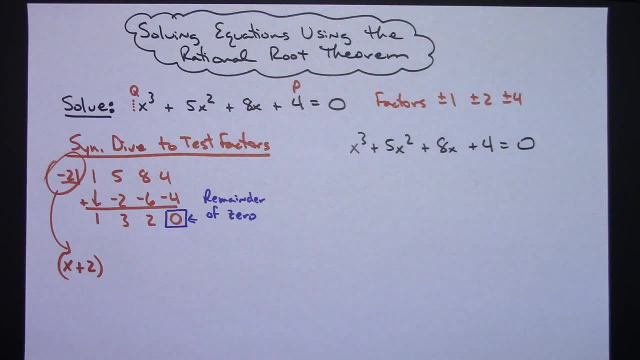 Alright, so I know one of the factors here is x plus two. Okay, now, where I come up with the rest of my factored form of this is going to be from the numbers that are right here. If you remember, in synthetic division this will be your constant. 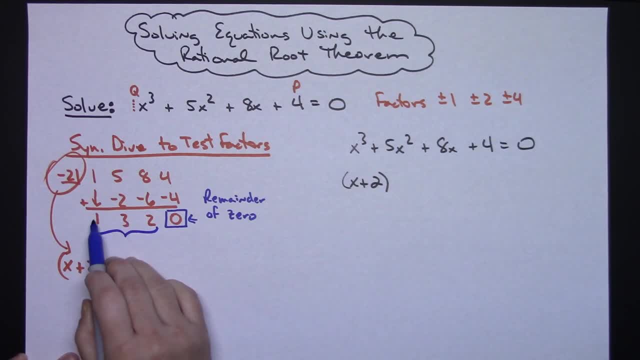 And then, because this is always a remainder, this is your constant, This is your x term. This would be an x squared term. If I had another number, it would be x to the third, x to the fourth, x to the fifth, and so on. 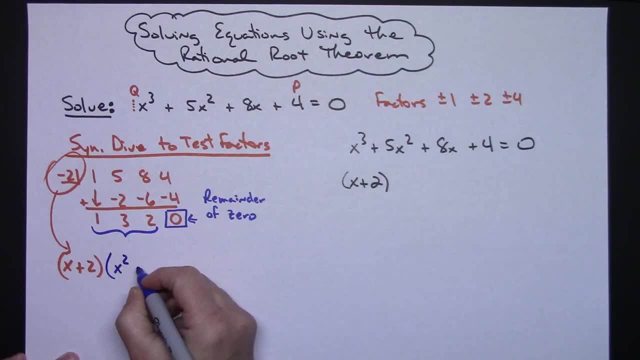 So from this I can come up with an x squared plus a three, x plus a two. Okay, so that means that my other factor over here is: x squared plus three, x plus two equals zero, And I've got two things there now that are multiplying together. alright, equals zero. 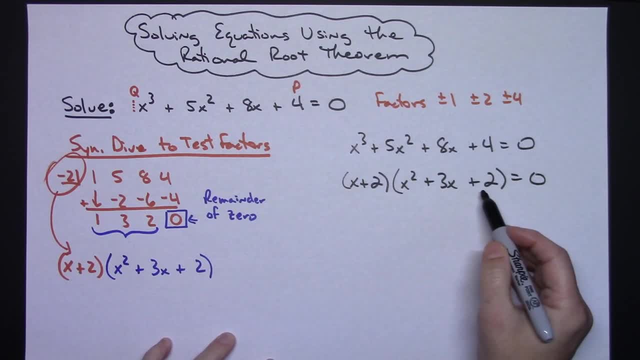 Now I can't do anything with this one, alright, but I can look at this and hopefully, at this point this is going to be a trinomial that we can factor yet again. So this x plus two is just going to stay x plus two. 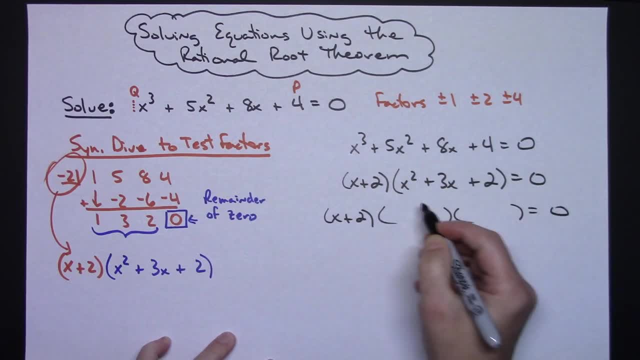 And then I'm going to see what I can play with here to factor this: Alright. so I know a leading coefficient, x, squared there. so x and x, Alright, Only things factors of two would be two and one. Everything is positive across the board. so I have to have a plus and I have to have a plus. 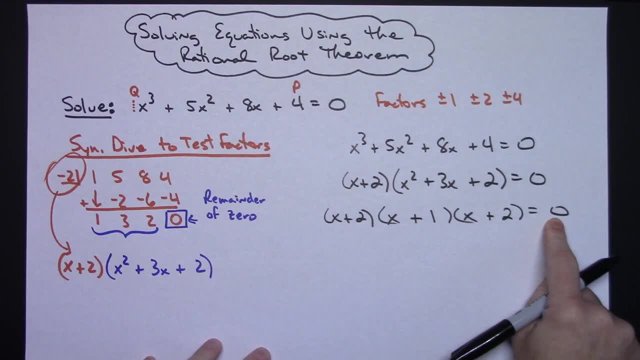 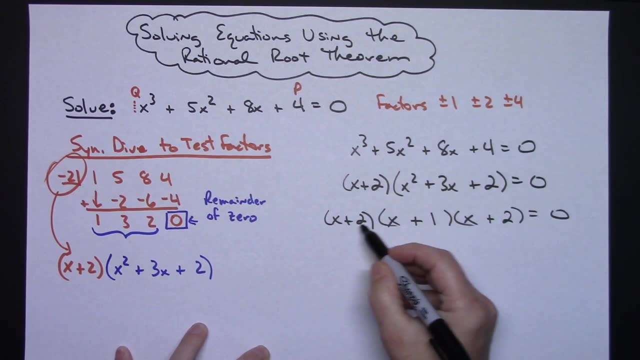 Alright, now I have completely factored this original equation with the rational root theorem and now I can use that zero product principle that says I can set each one of these equal to zero and solve. So x plus two equals zero. so x equals negative two. 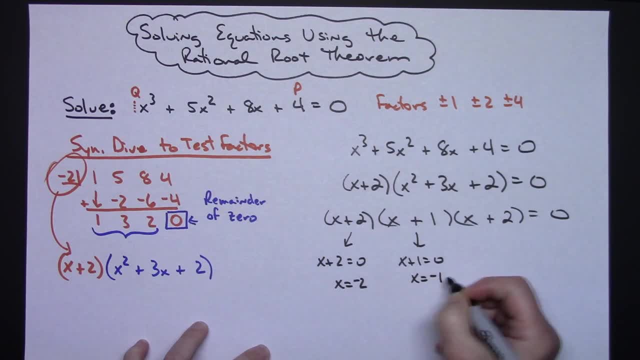 X plus one equals zero, so x equals Negative one. And then here I'm going to get the exact same thing: X plus two equals zero, so x equals negative two. Alright, so my solutions are negative two and negative one. if you need to write it as a solution set. 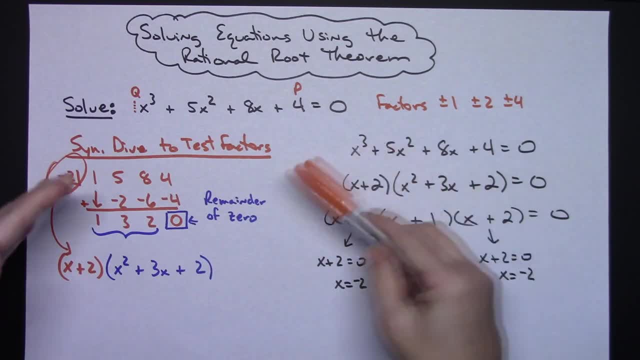 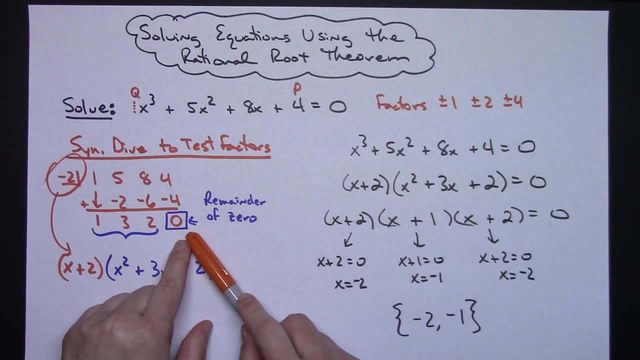 Alright, now, I did do this one and in the guess and check process of checking all these factors, I did pick one and it became a factor right away. I got you know, I got lucky. Your thing is you're.